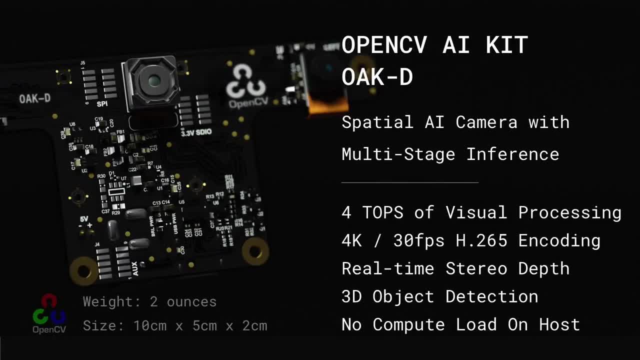 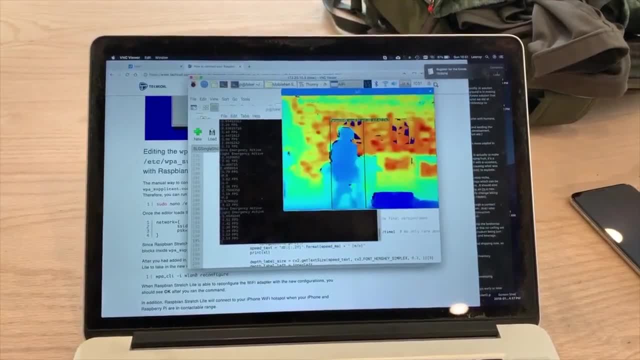 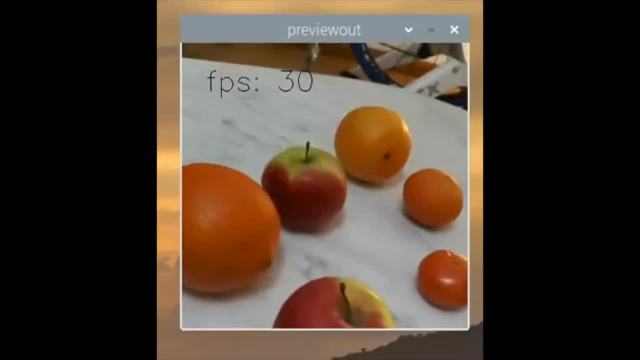 And Oak D ups the ante with stereo cameras for 3D depth capabilities. Depth perception with artificial intelligence is like a cheat mode for solving all sorts of problems. Out of the box, Oak comes with incredibly powerful neural networks that allow developers to detect and track almost anything in 2D and 3D space. 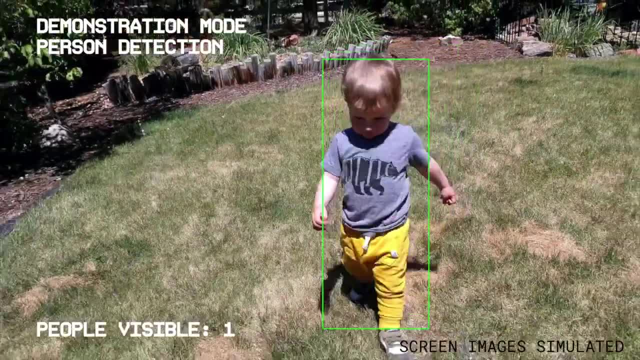 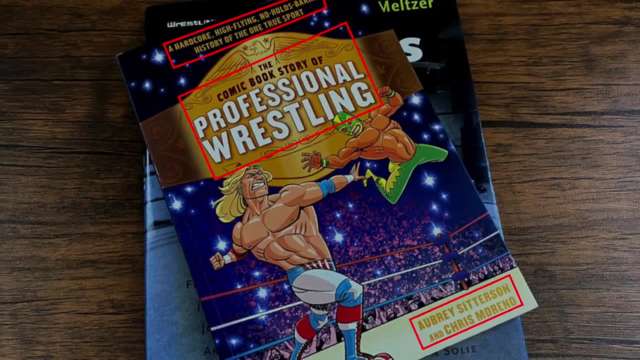 With a few lines of code, you can run multi-stage processing and pass off detection and re-identification results to other included networks, such as visual estimation, facial landmark detection, optical character recognition and semantic segmentation. You can even use free online tools to train your own networks. 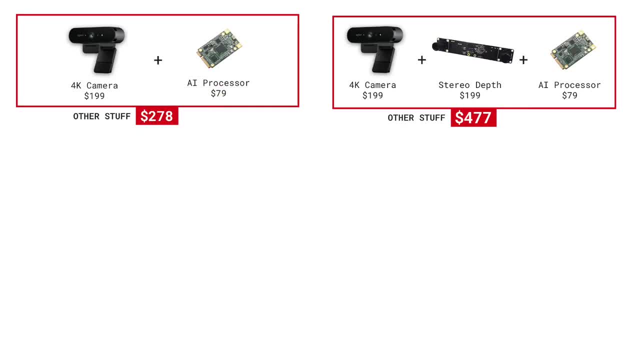 Not only that, the OpenCV AI Kit is the most affordable complete spatial AI system in the world. In fact, many of the individual components would cost more than either Oak One or Oak D during this campaign. That's right. it's not a typo. 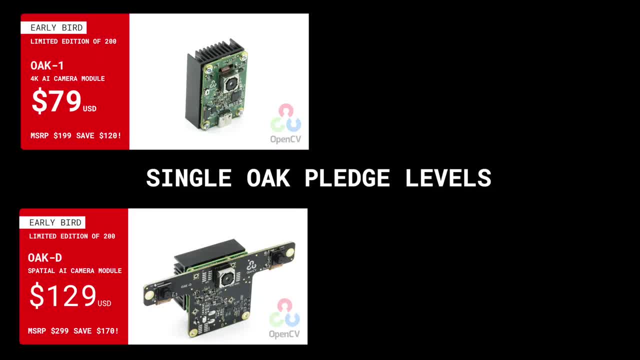 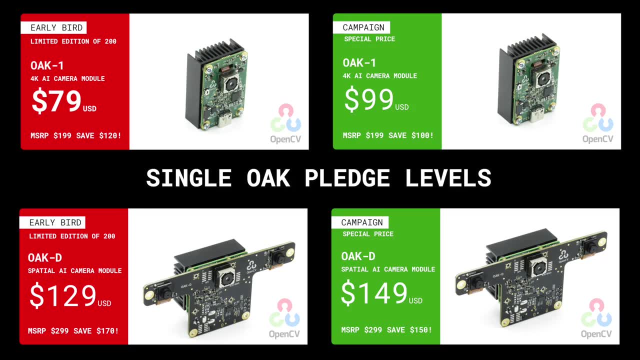 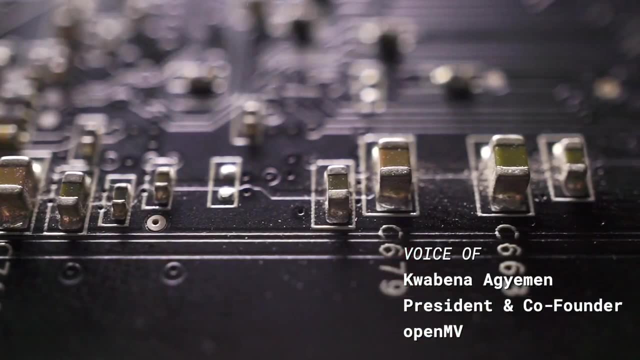 Oak One is just $79 and Oak D just $129 for early birds. Regular campaign prices are $99 and $149, which is still a savings of 50% off MSRP. With OpenCV AI Kit, you can finally build a product using Myriad X, which is huge. 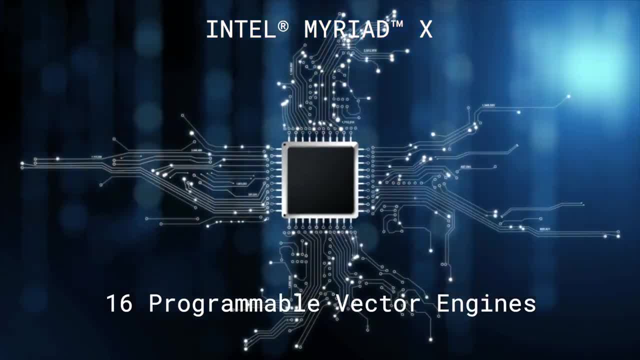 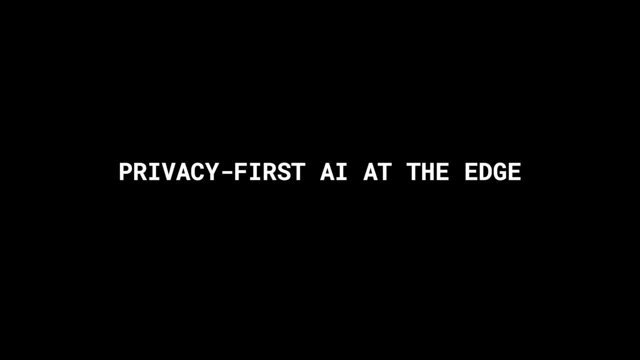 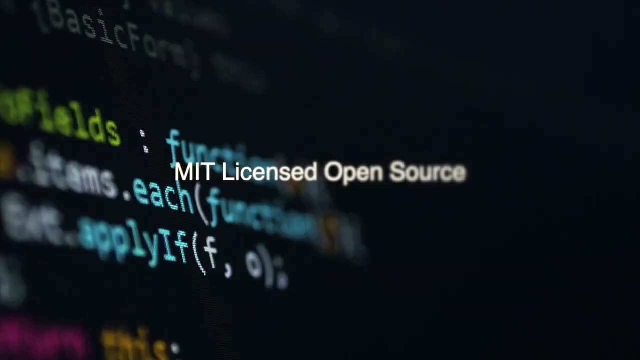 The backbone of OAK's advanced features is the Myriad X. This powerful VPU leaves your host operating system completely free for other business logic. Since OAK runs artificial intelligence locally, there's no need for a cloud upload. Since it's open source, you can see everything OAK does. 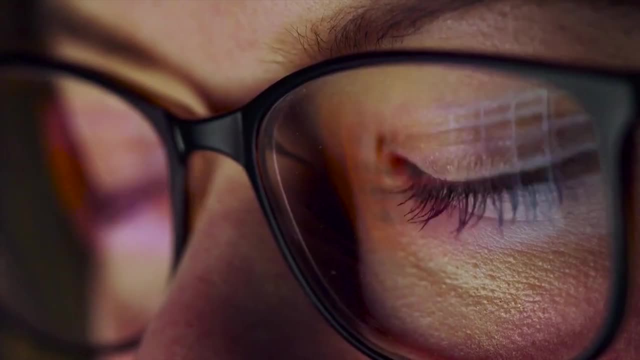 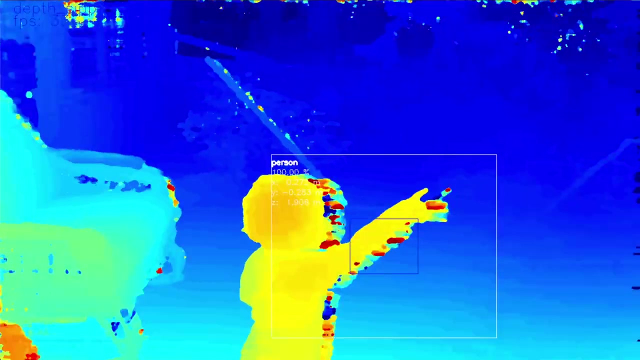 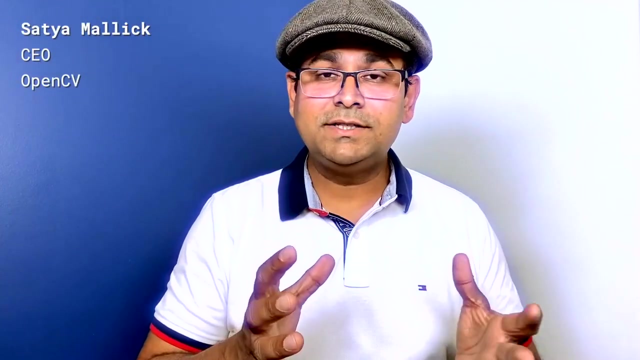 With great power comes a great programming interface. The OAK API, in addition to OpenCV, allows for beginner-level control of both these boards, but also allows much deeper access for professional implementations. This is not just a good camera for companies who are trying to build smart cameras. 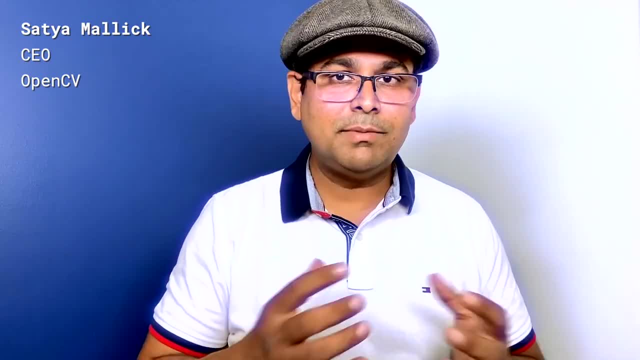 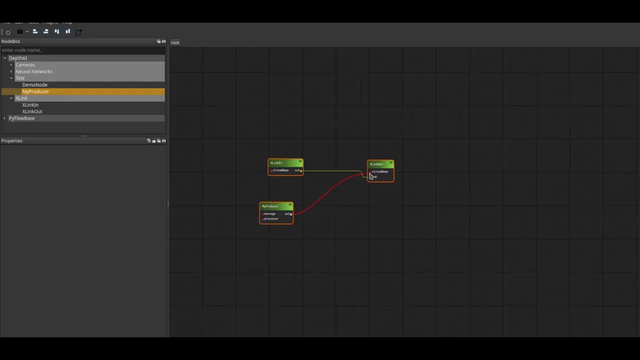 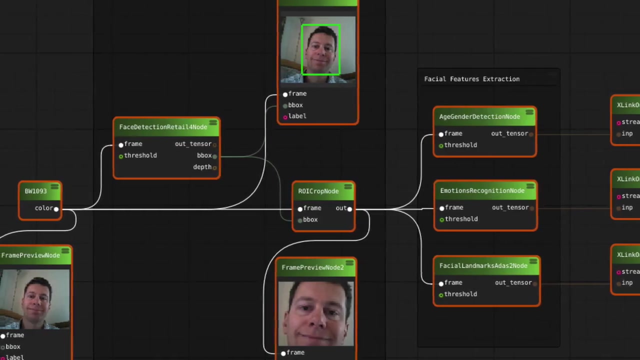 It is a great camera for people who want to learn about spatial AI and edge AI. OAK also brings a new visual pipeline builder. Arrange computer vision and AI workflows using a node-based editor that includes previews, so you can be sure your inferences and CV functions are behaving as expected. 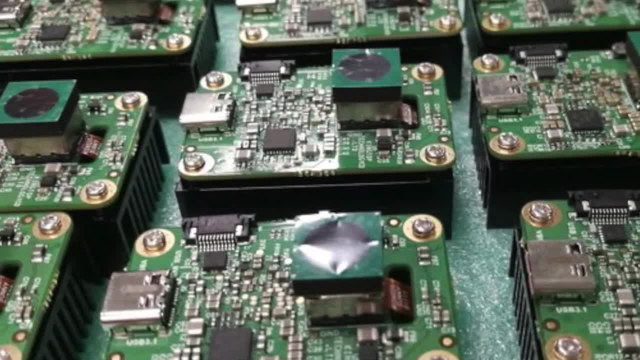 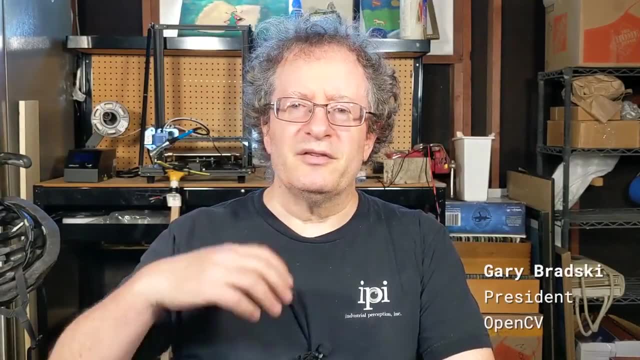 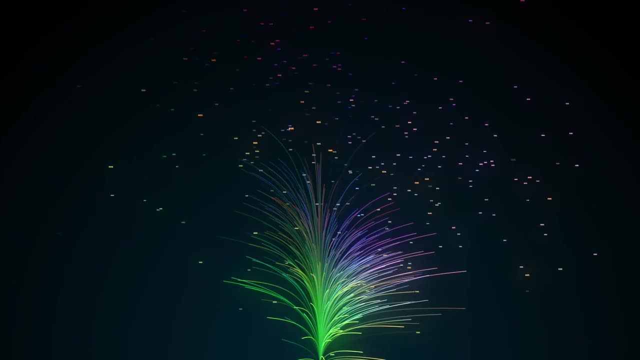 Oak One and Oak D are both FCC and CE certified and were built with an easy path to productization in mind. Research papers, contests, robotics, startups: we want to see it Blow us away. Twenty years ago, combining computer vision and artificial intelligence was barely an idea. 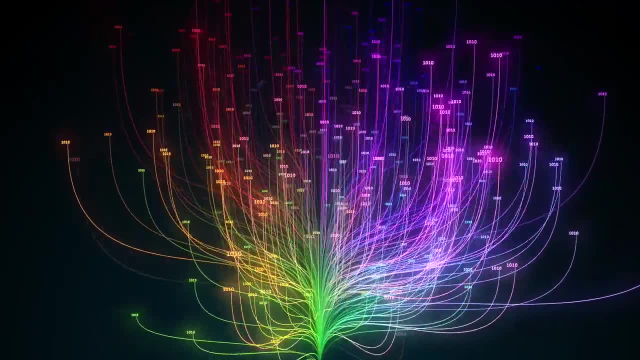 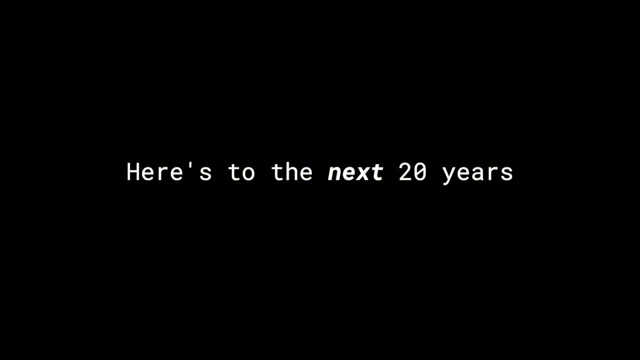 With the OpenCV AI kit. it's an idea you can hold in your hand and combine with your own ideas to make something brand new. We can't wait to see what you do with it. For more information, visit wwwoakedu. 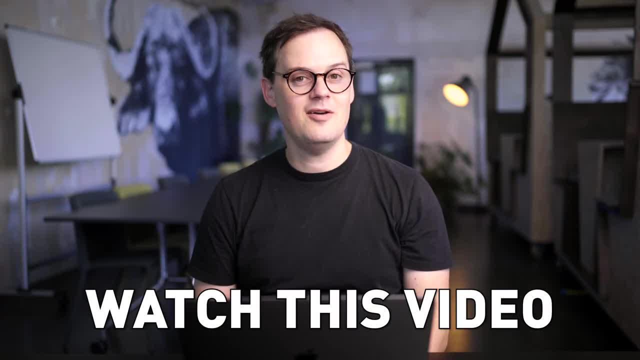 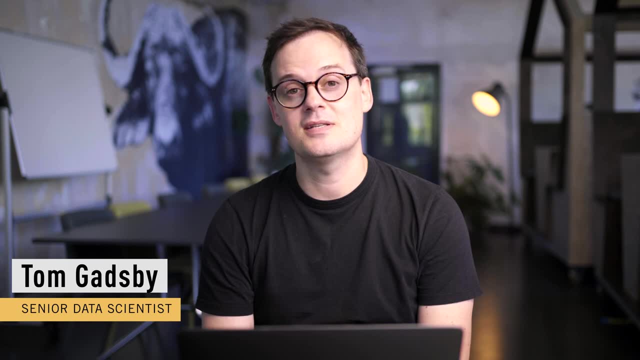 Have you read articles about how cool it is to be a data analyst? Watch this video and find out if it suits you. My name's Tom. I've been working in the field for more than five years and I'm currently a senior data scientist at Career Foundry. Data analyst is one of the hottest job. 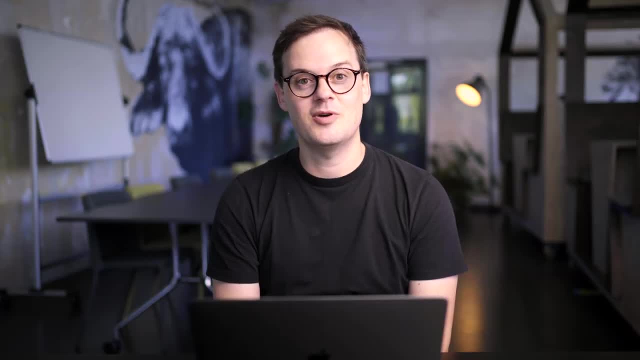 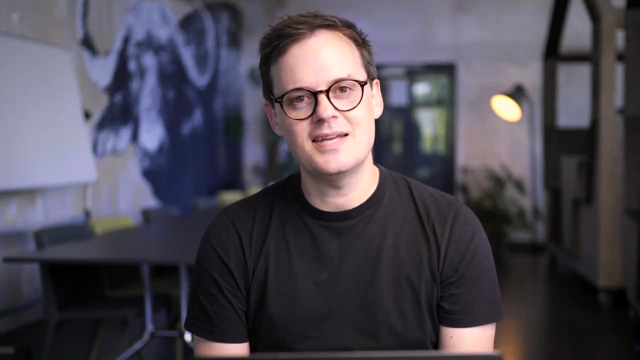 titles in 2022.. A job in data promises exciting career prospects, so it's no surprise that more and more people are transitioning into the field, and with the demand comes great salaries. So what does it take to thrive in this industry and how do you know if it's the right career for you? Career. 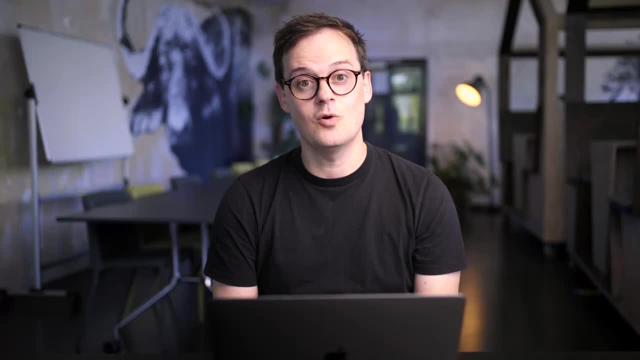 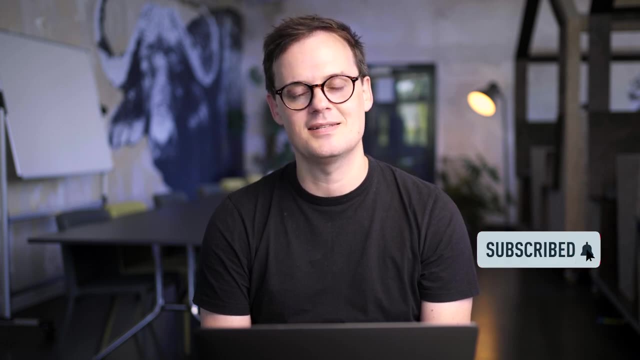 change isn't easy, and it's not just about salary and job title. You also have to love what you're going to do and be good at it. So in this video, we'll help you figure out if you have what it takes to be a good data analyst and, more importantly, whether a career in data analytics 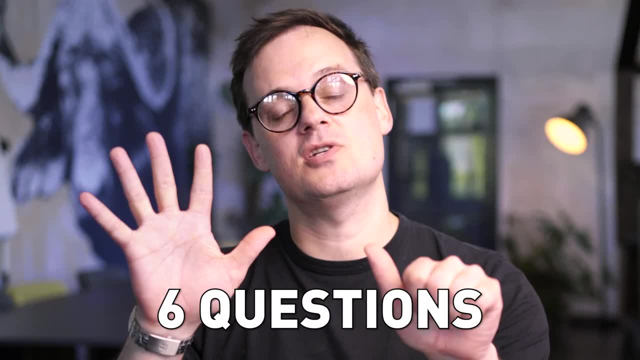 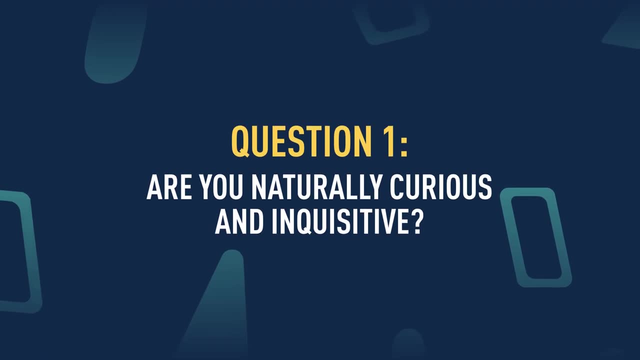 aligns with your own goals and objectives? Here are six questions you'll need to ask yourself before starting a career in data analytics. So let's start with question number one. Are you naturally curious and inquisitive? Analytics is about trying to find insights from data. 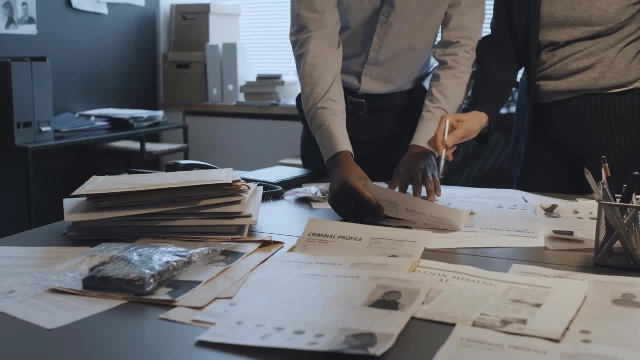 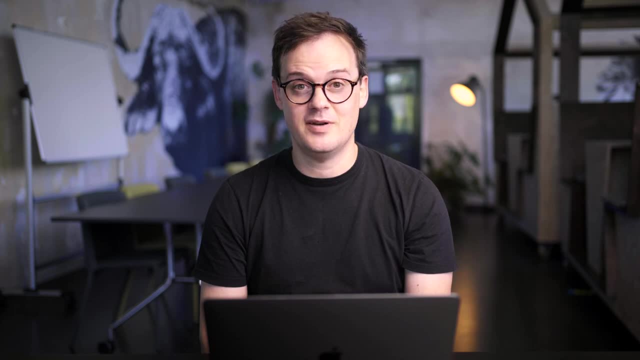 Think of yourself like a data detective. And just like detectives, clues in the data are often hidden where other people haven't thought to look. You will need to work hard and dig deep into the data to find insights. This means you'll be operating in uncertainty A lot of the time. you'll be working by yourself. Are you comfortable? 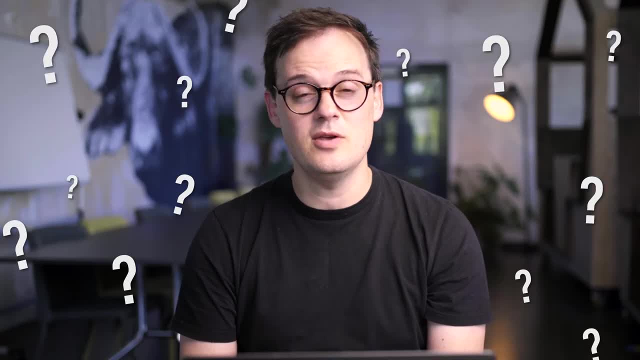 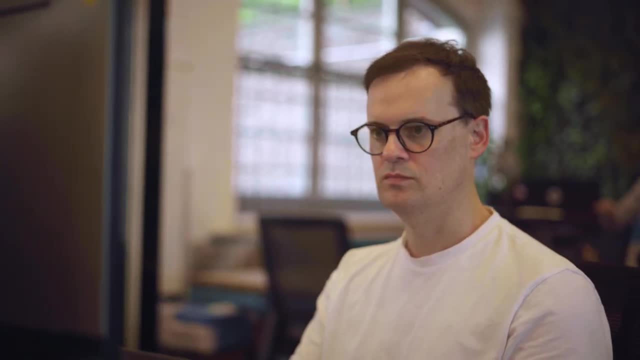 working in uncertainty and admitting to yourself you don't really know where you need to go. You will also make a lot of mistakes. Finding new insights involves trial and error. Are you confident in your ability to solve something despite having failed at it four or five times previously? Check?